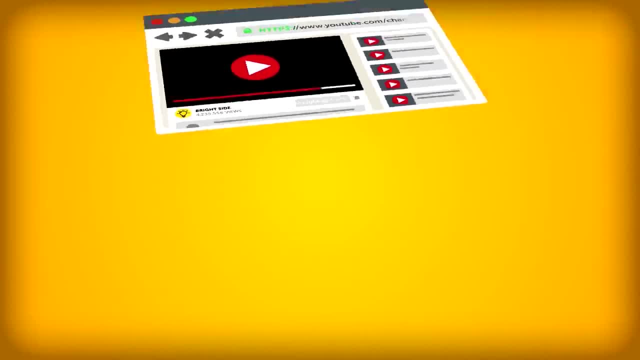 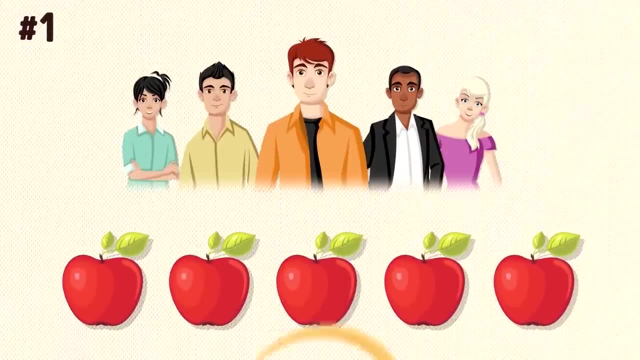 Stay on the Bright Side. 1. Okay, let's start with an easy one. You have five apples in a basket and five people to distribute them to. How can you give an apple to each person while still leaving one in the basket? 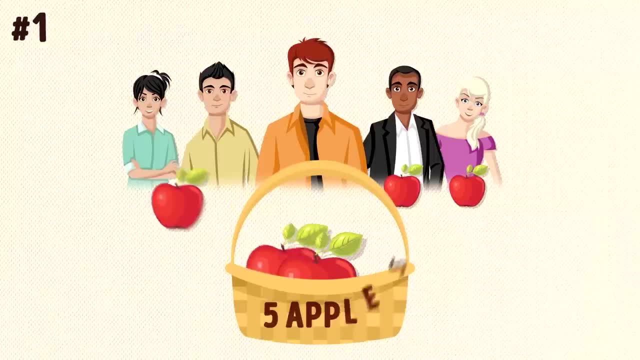 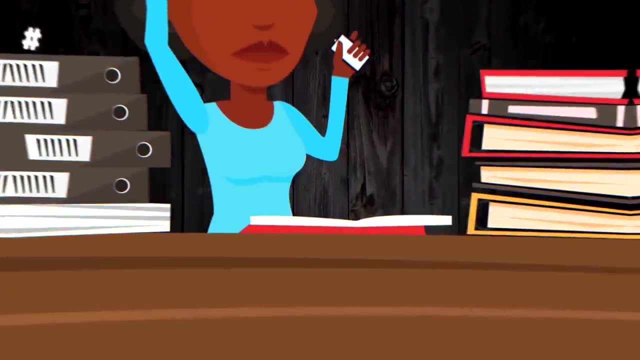 Does your head hurt? yet The answer is actually pretty simple: Just keep the last apple in the basket and hand the basket with the apple in it to the fifth person. 2. Listen carefully to these words. Imagine you're in an office building. 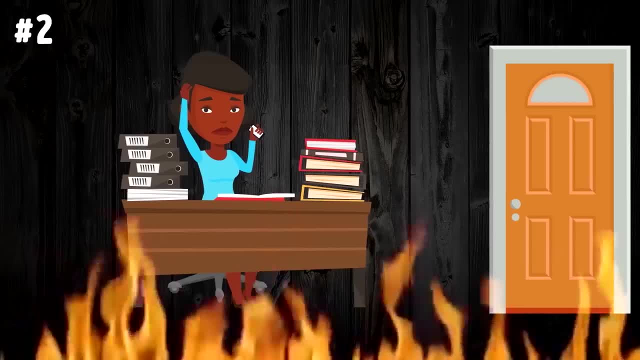 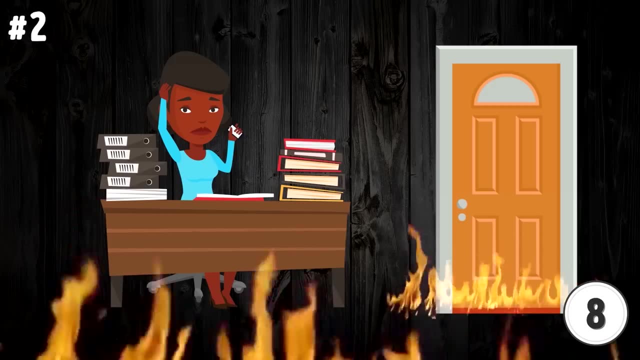 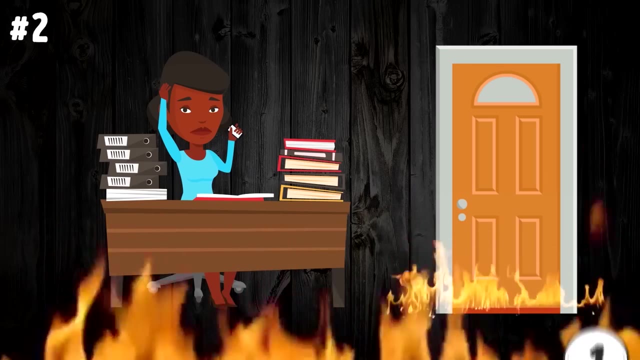 and everything around you is on fire. Just beyond the desk in front of you is a door, but flames are in front of it. How do you get out The answer? Well, stop imagining. The beginning of the sentence was imagine. 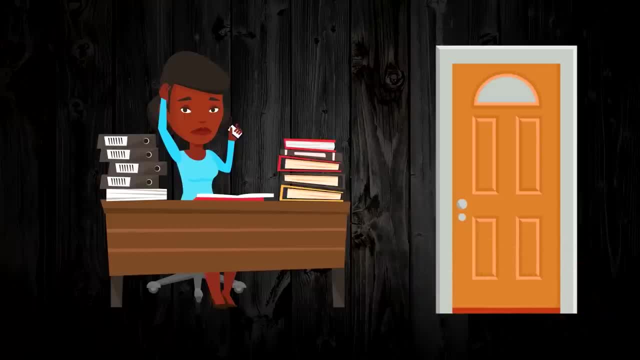 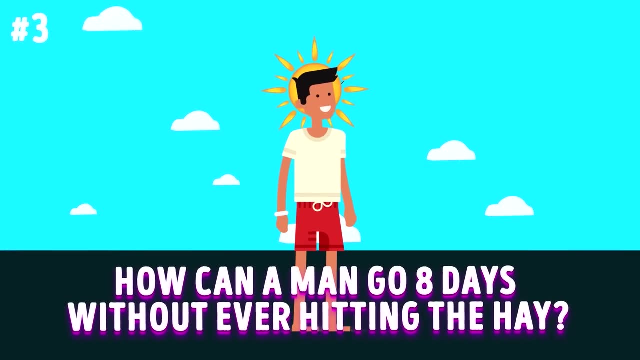 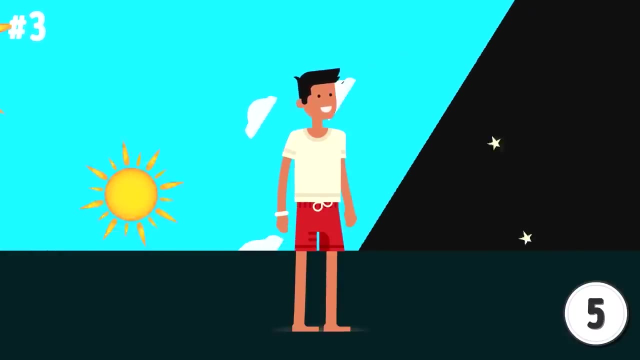 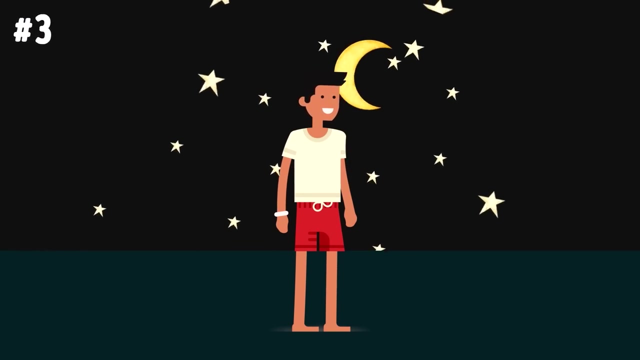 Imagine you're in an office building, So the scenario wasn't even real in the first place. You were just imagining it. 3. How can a man go eight days without ever hitting the hay The same way you do? He sleeps at night. The same answer would apply, conversely. 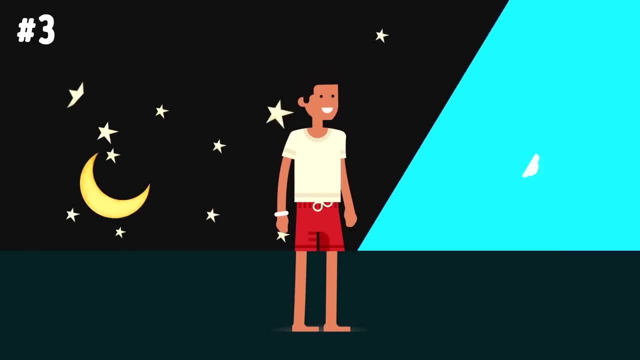 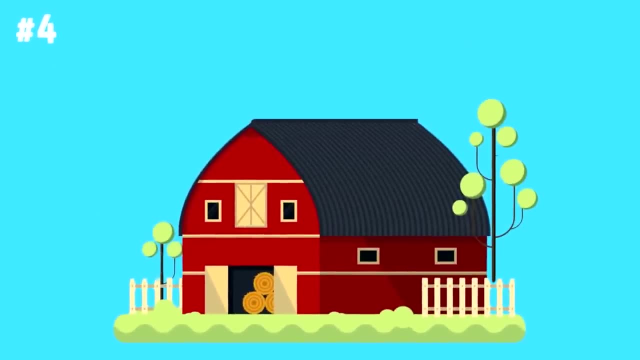 If a man can go eight nights without sleep, it's probably because he slept during the day. Pretty tricky, right? 4. Picture this: You live in a barn While standing on the barn roof with one of your roosters. 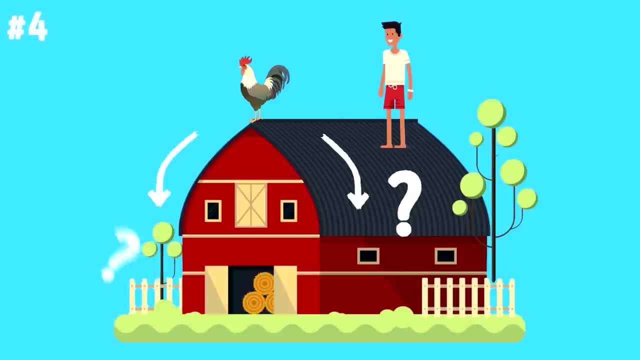 it lays an egg. In which direction does the egg roll? Um, the egg doesn't roll anywhere. because the egg is in the barn, Because there is no egg. Roosters don't lay eggs. Perhaps the bigger question is: why are you guys on the barn roof? 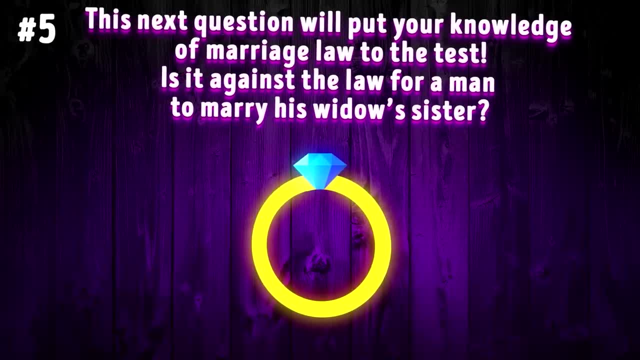 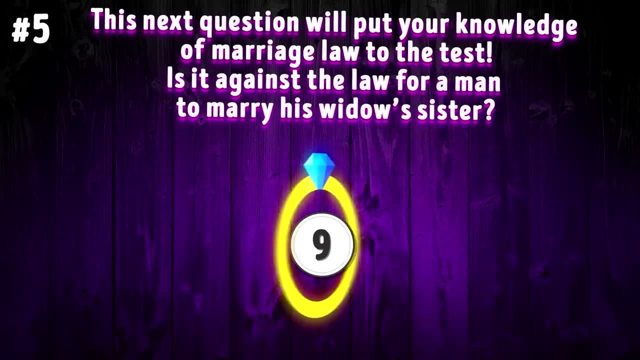 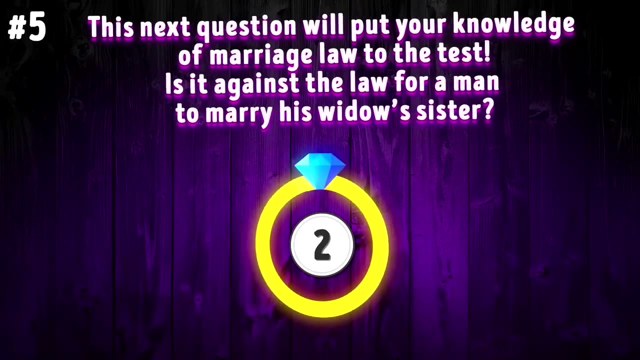 5. This next question will put your knowledge of marriage law to the test. Is it against the law for a man to marry his widow's sister, While it's not exactly illegal? 5. This next question will put your knowledge of marriage law to the test. Is it against the law for a man to marry his widow's sister? 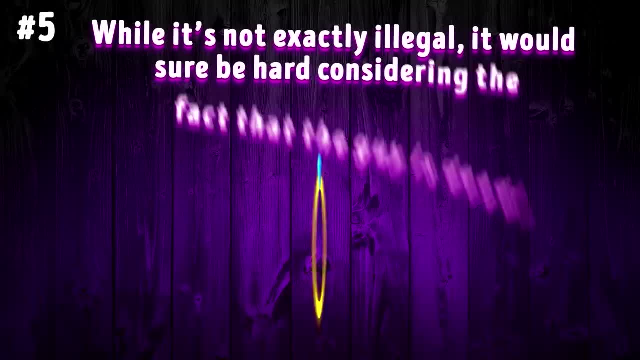 While it's not exactly illegal. 6.. This next question will put your knowledge of marriage law to the test. Is it against the law for a man to marry his widow's sister? It would sure be hard, considering the fact that the guy is dead. 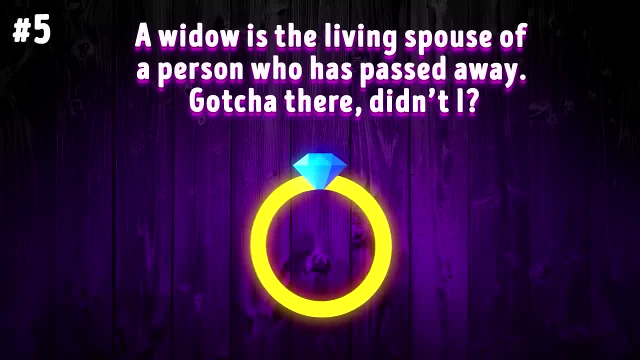 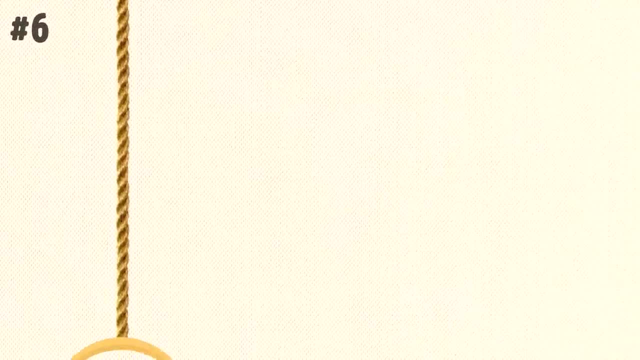 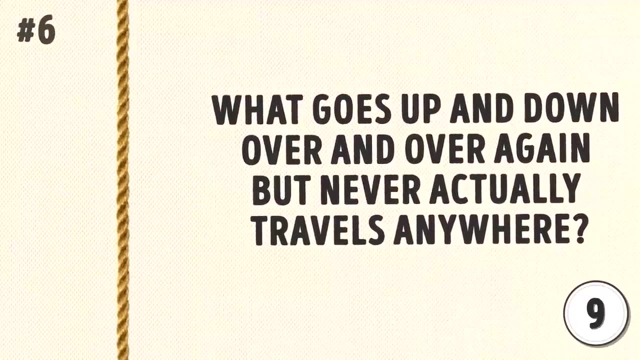 A widow is the living spouse of a person who has passed away. Got you there, didn't I? 6. You may have to really rack your brain with this next question: What goes up and down over and over again but never actually travels anywhere? 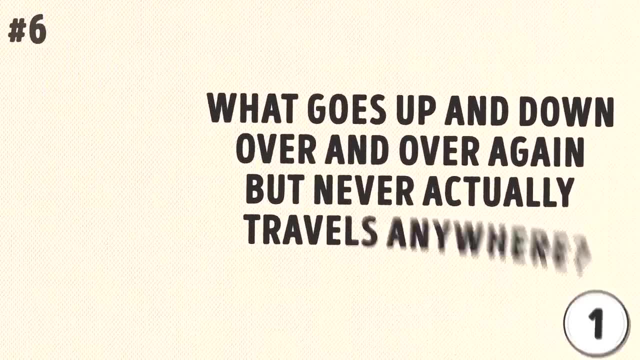 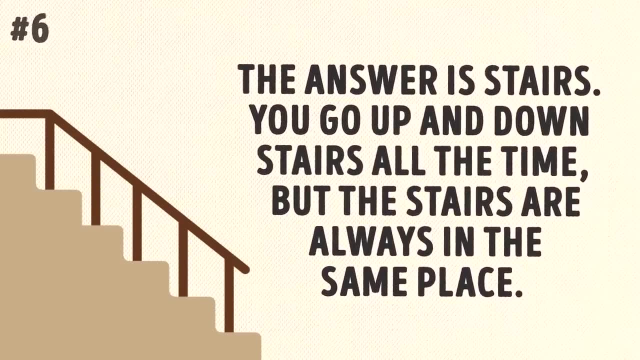 7. What goes up and down over and over again, but never actually travels anywhere? What goes up and down over and over again, but never actually travels anywhere? Do you give up? The answer is stairs. You go up and down stairs all the time, but the stairs are always in the same place. 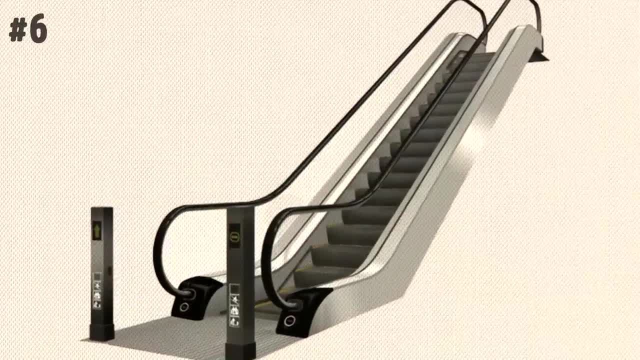 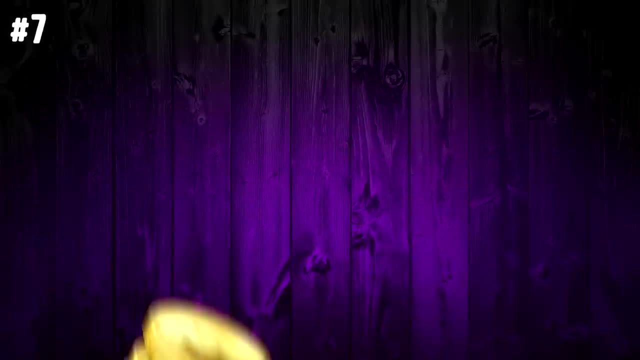 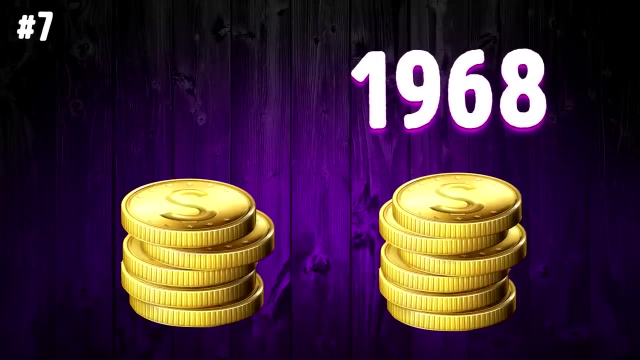 Unless, of course, you're talking about escalators, which are moving stairs. Okay, things are getting a little complicated here. 7. You'll love this question. It's all about money, honey. Do you know why 1968 pennies are more valuable than 1967 pennies? 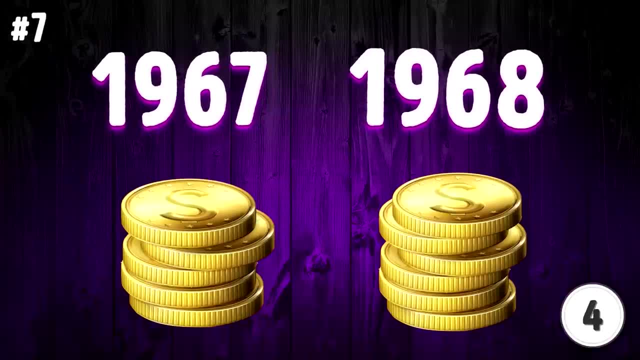 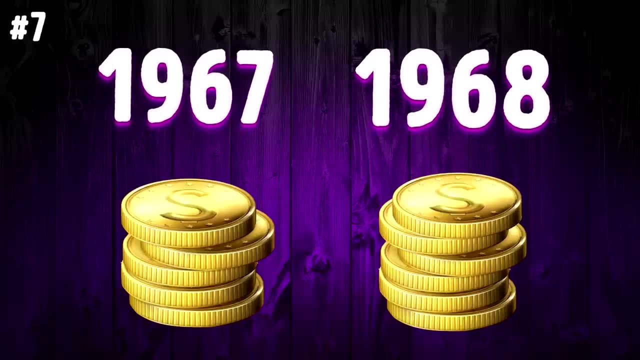 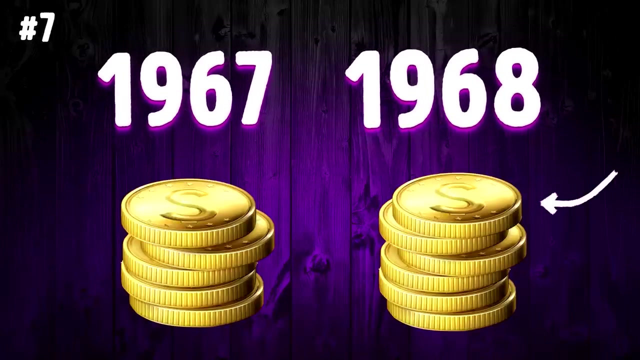 Well, considering the fact that 1968 is just one digit higher than 1967, that makes the amount larger and therefore a smidge more valuable. The numbers are referencing the amount of pennies and not the year, like your brain probably thought. 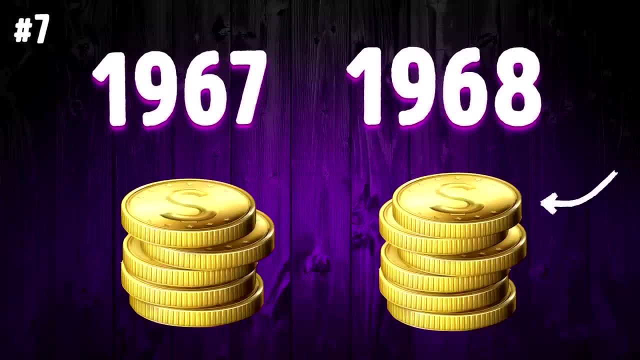 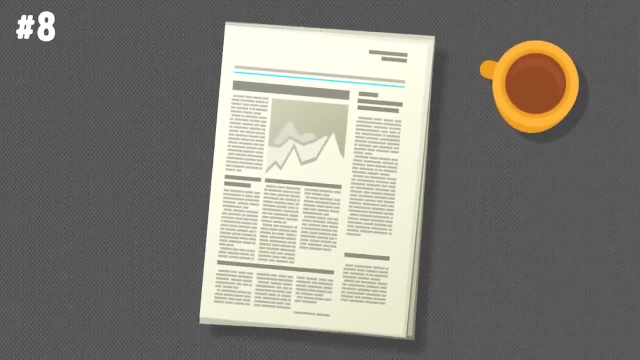 Generally, no matter what year pennies were manufactured, they're all the same value. 7. What goes up and down over and over again but never actually travels anywhere, One cent 8. Okay, you're all done reading the morning newspaper. 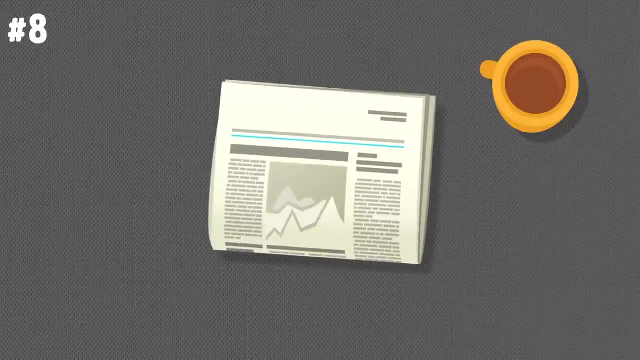 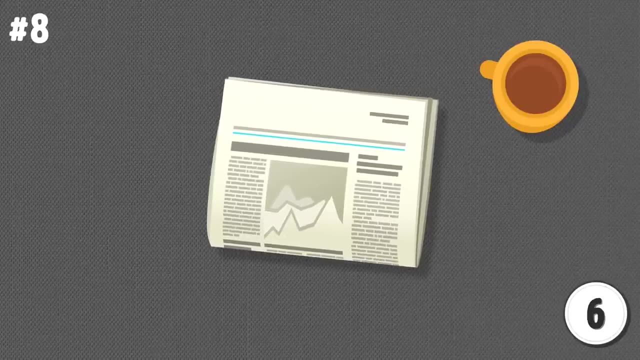 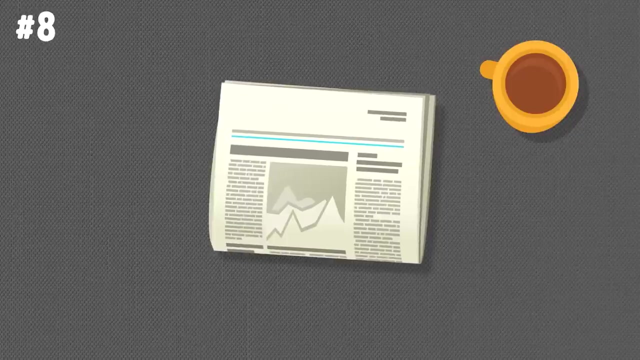 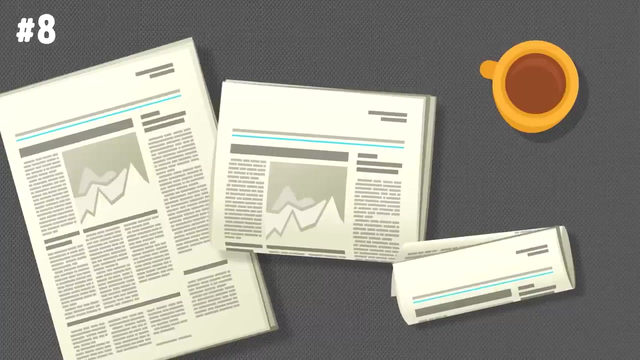 You take out one page and fold it in half. How many more times can you fold it in half? Can't come up with an answer. Well, you can technically only fold the paper in half once. If you continue, you'll be folding it into fourths, then eighths, then sixteenths. then you get the idea. 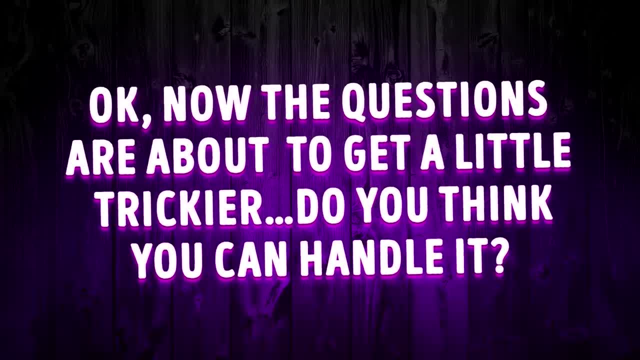 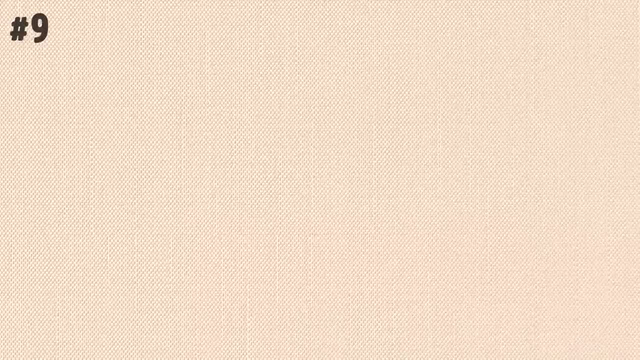 Okay, now the questions are about to get a little trickier. Do you think you can handle it? Let's put your common sense to the test. 9. This is Tom. Tom's dad has five sons named 10,, 20,, 30, and 40. 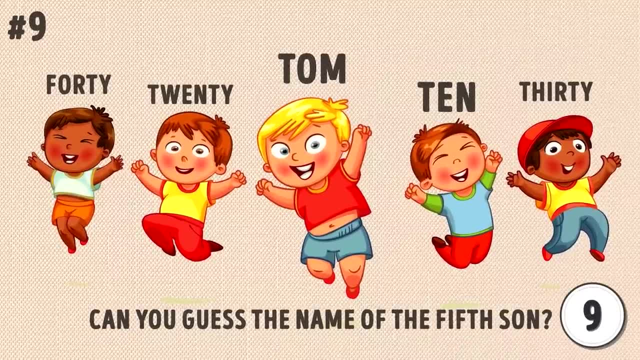 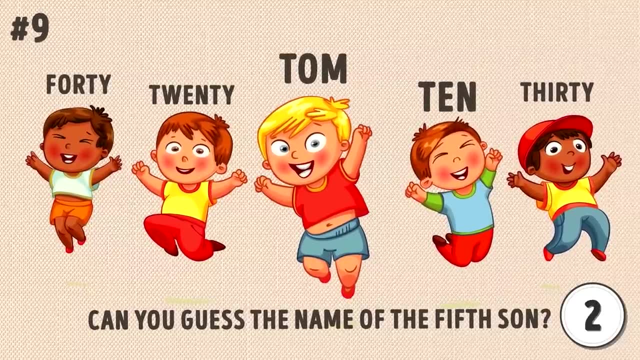 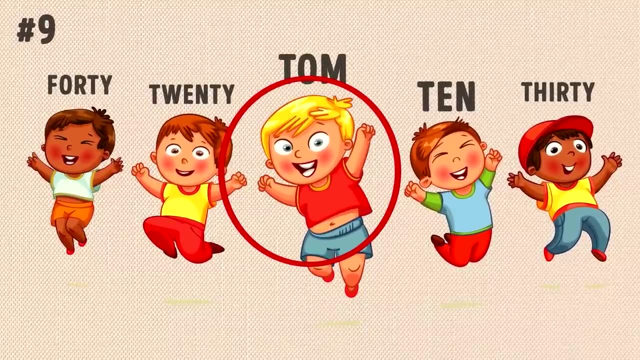 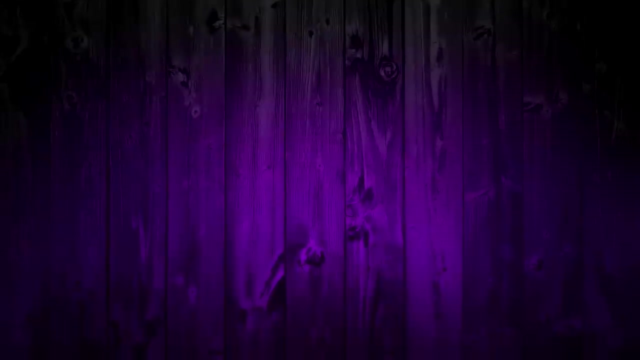 Can you guess the name of the fifth son? Are there more than one son in the family? Close your eyes. The answer was right in the question. The fifth son's name is Tom. The question said Tom's dad. After naming four of the sons, the fifth one must be Tom. 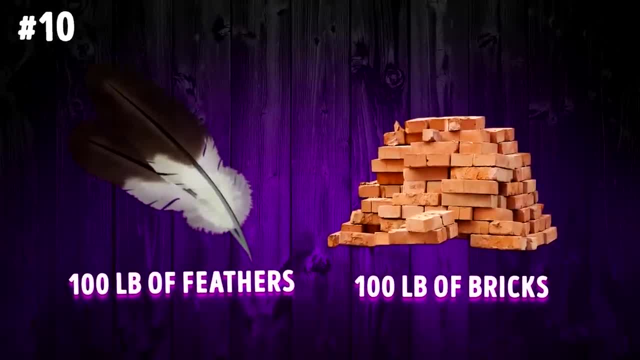 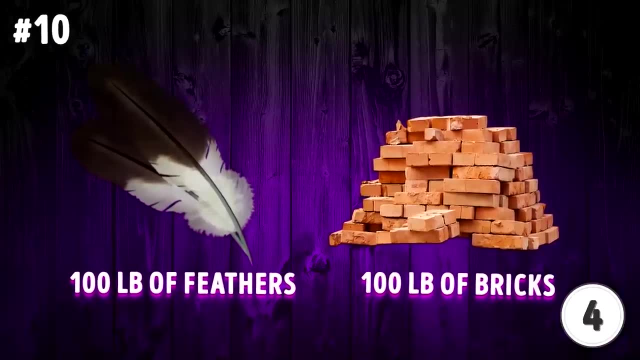 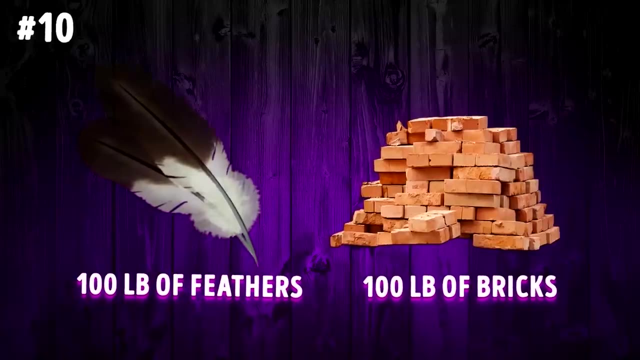 He spread his name just like this: 10.. What weighs more, 100 pounds of feathers or 100 pounds of bricks? You're probably assuming bricks, since they're obviously much heavier than feathers, But if you look a little closer at this question, you'll see that the answer is right there. 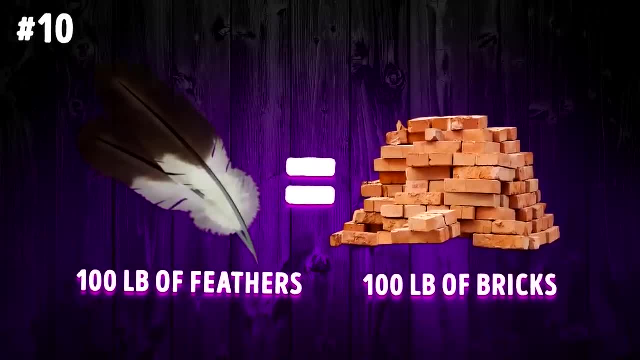 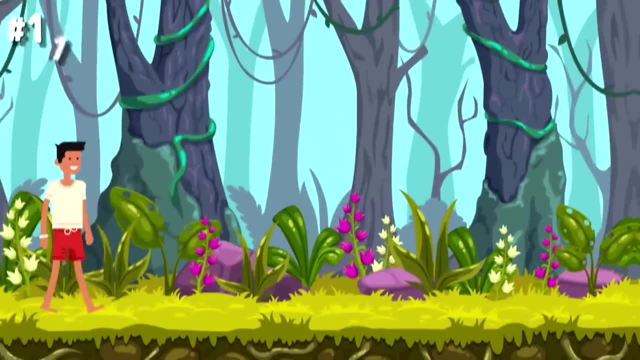 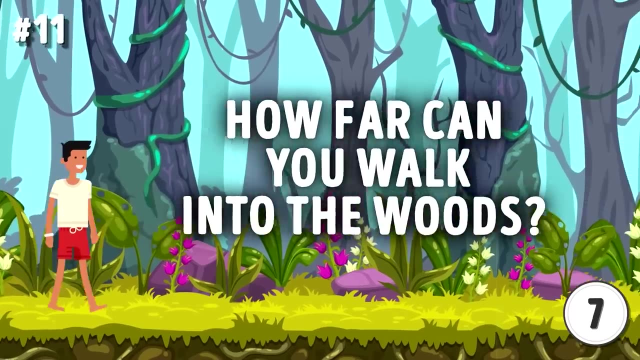 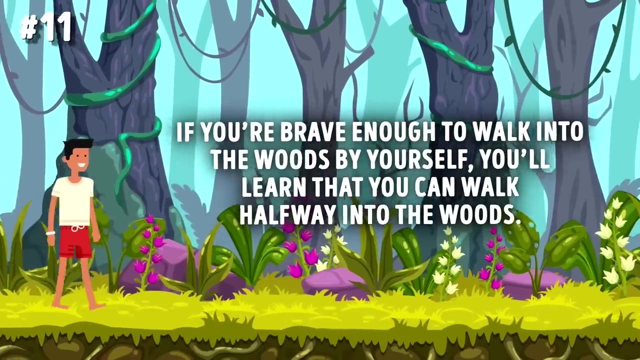 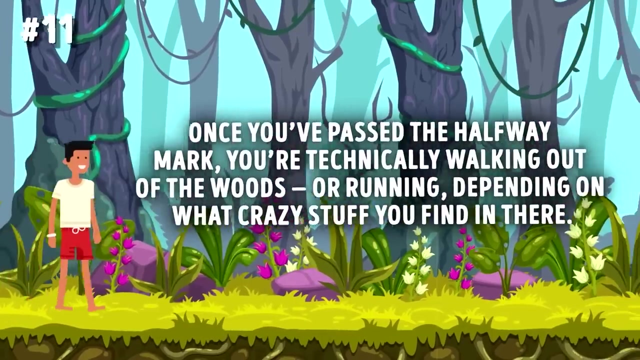 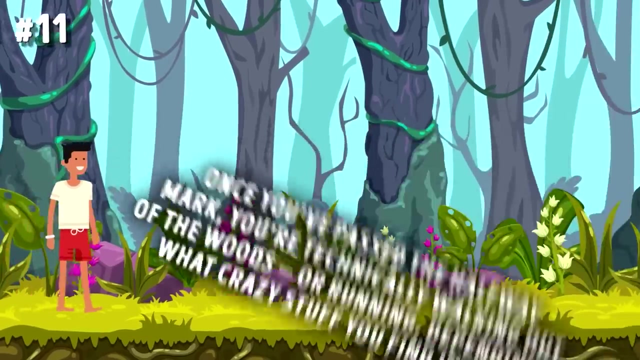 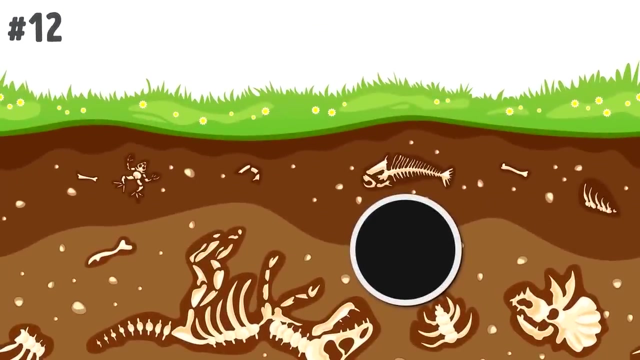 Both the feathers and the bricks weigh 100 pounds. It's the amount of feathers and bricks that vary, not their weight of 100 pounds. 11. How far can you walk into the woods? 12. Think you're a whiz at math. Let's see if you can answer this question. 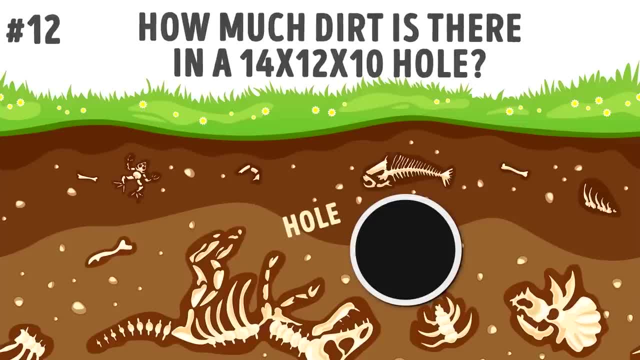 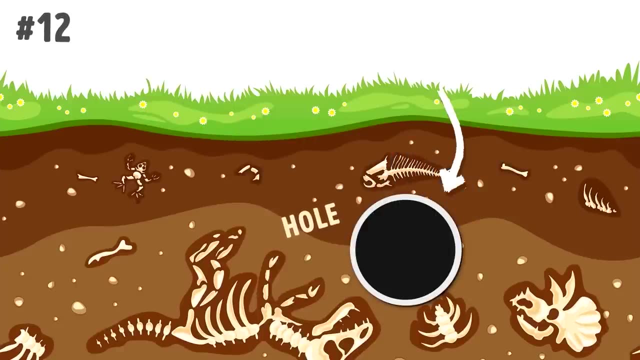 How much dirt is there in a 14x12x10 hole? Okay, before you get a headache from all that computing, I'll give you the answer. There isn't any dirt in the hole. If it were filled with dirt, or anything for that matter, it wouldn't really be a hole, would it? 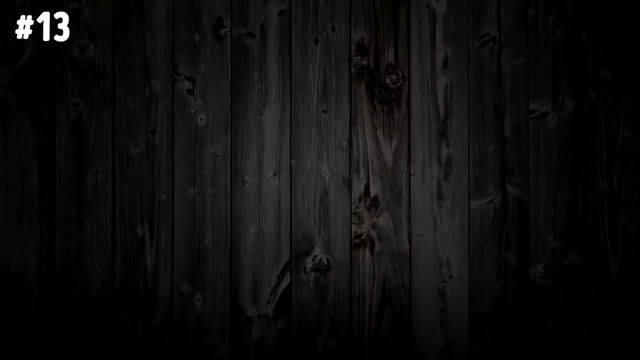 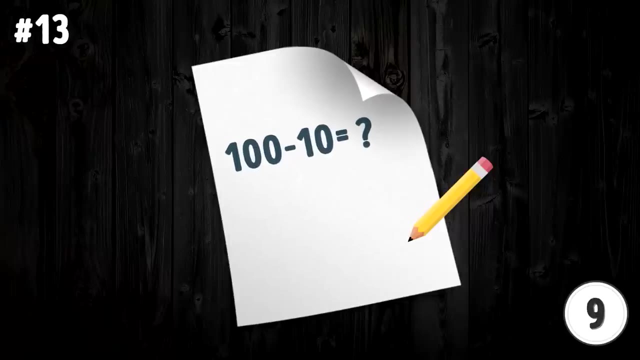 13.. Here's another math question. Another math question for all you wannabe Einsteins out there: How many times can you subtract 10 from 100?? Okay, let's walk through this one together. If you were to subtract 10 from 100, you'd end up with 90.. 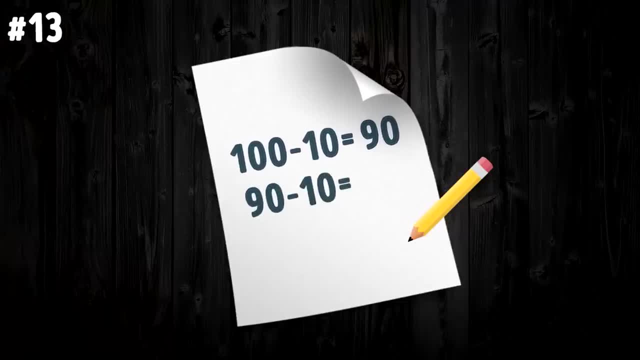 So if you subtracted 10 again, well, you wouldn't be taking it from 100.. You'd be taking it from 90.. If you took away 10 more, you'd be taking it from the new amount of 80.. 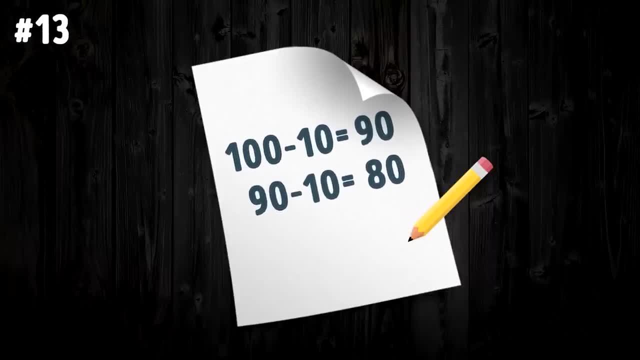 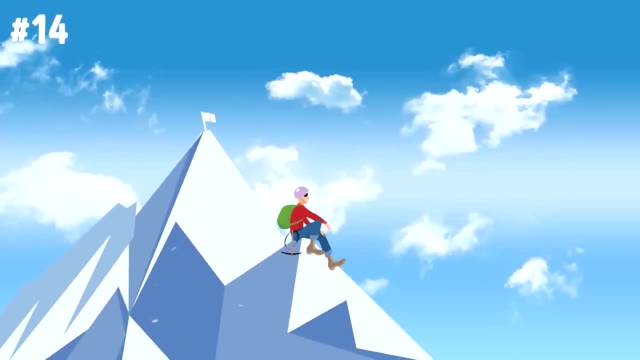 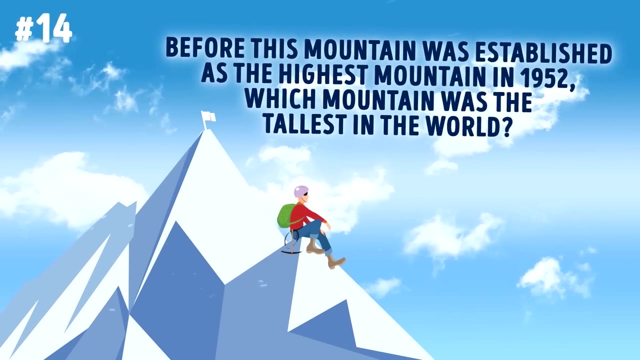 This means you can only subtract 10 from 100. once Makes sense, right 14.. You know how Mount Everest is the tallest mountain in the world, right Well before this mountain was established as the highest mountain in 1952,. 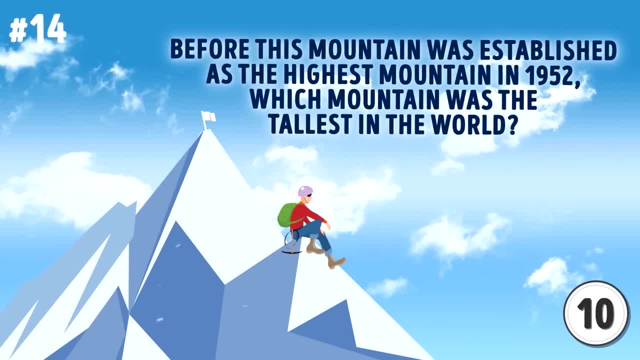 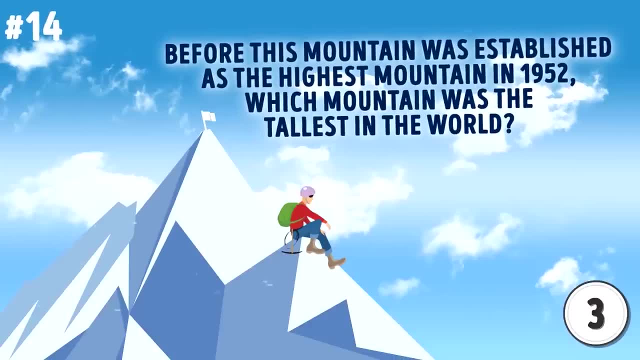 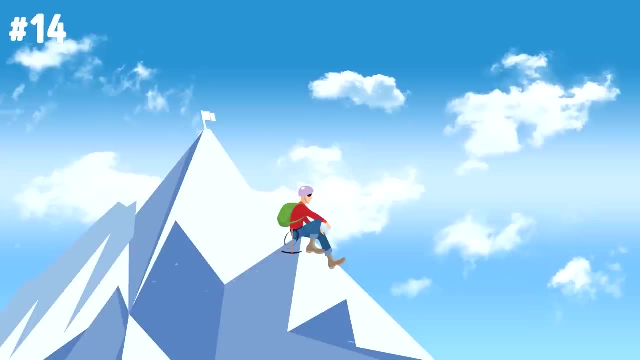 which mountain was the tallest in the world? 15. Mount Everest is the tallest mountain in the world today. It was the tallest 100 years ago, 200 years ago and so on. Racking your brain, trying to remember what you learned in geography class back in high school. 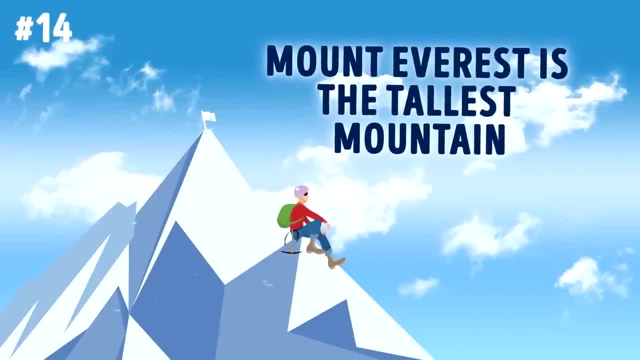 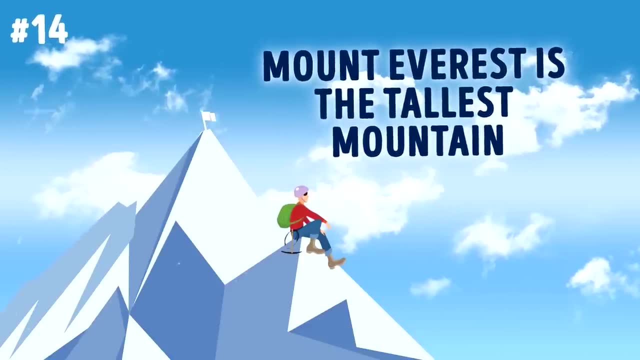 Well, you're wasting your time. If Mount Everest is the tallest mountain in the world today, it was the tallest 100 years ago, 200 years ago and so on. It still existed here on Earth. We just didn't know it yet. 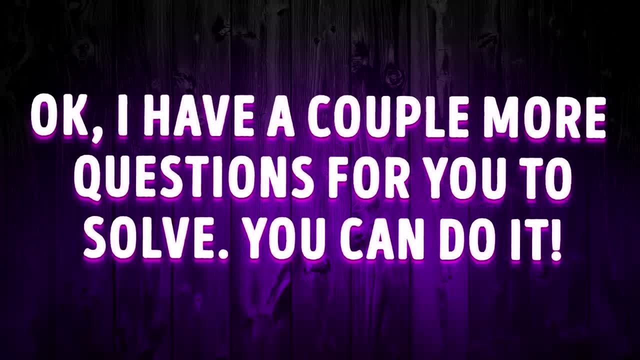 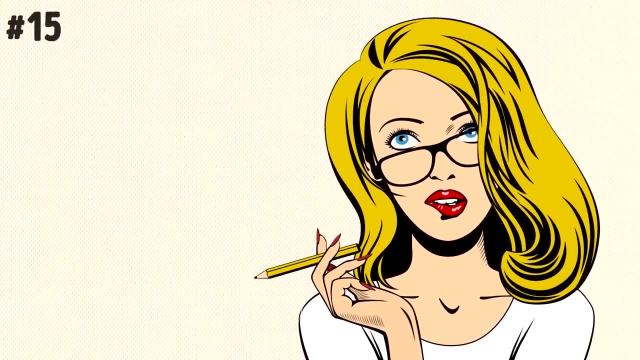 Still hanging in there. Okay, I have a couple more questions for you to solve. You can do it 15.. Think you're a wordsmith, do ya? Let's try this question on for size: Which word becomes shorter after adding two letters to it? 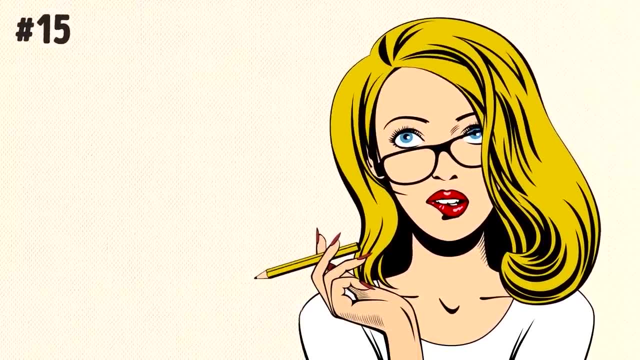 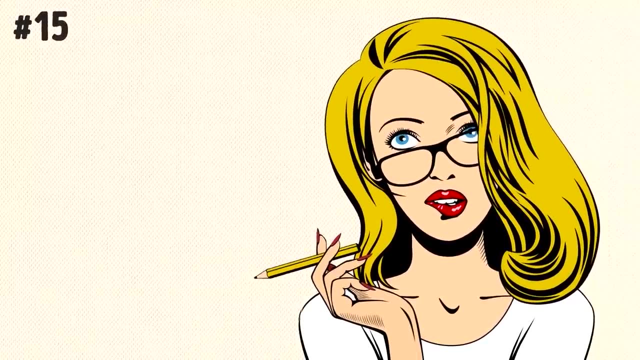 Wait a minute. How can a word become shorter if you're adding letters to it? That doesn't make any sense. Actually, it makes plenty of sense once you realize. the word I'm talking about is short If you add two letters to the word. 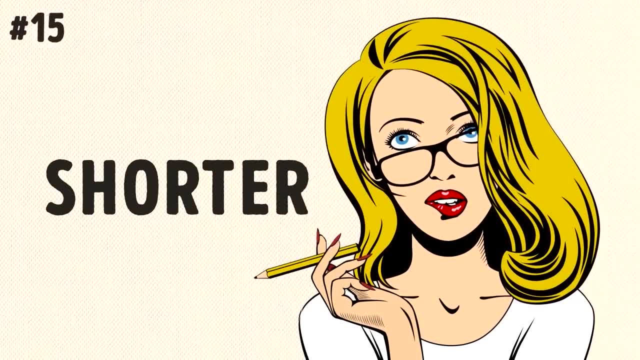 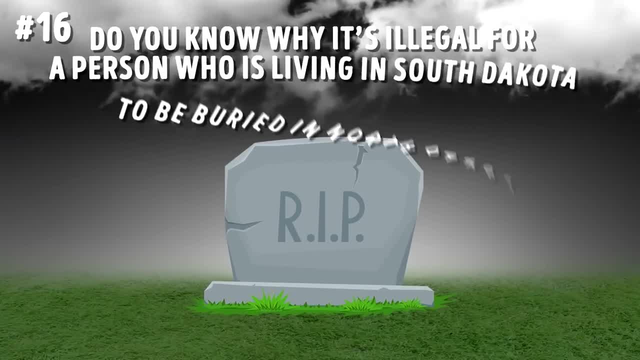 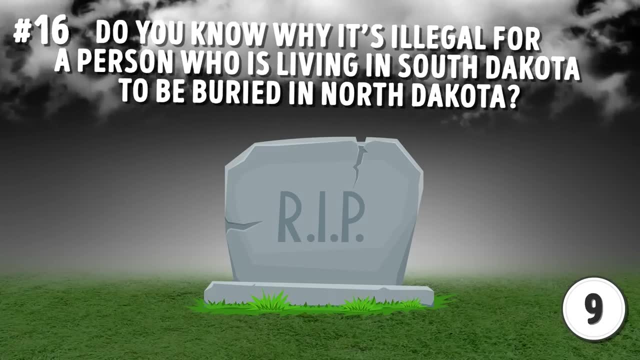 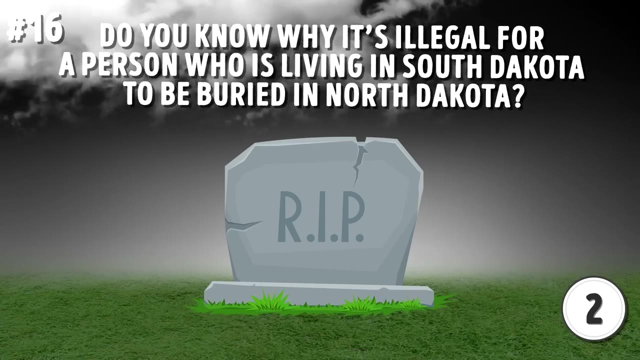 specifically E and R. the word literally becomes shorter. See, it does make sense. 16. Do you know why it is illegal for a person who is living in South Dakota to be buried in North Dakota? Um, you know that burying a person alive 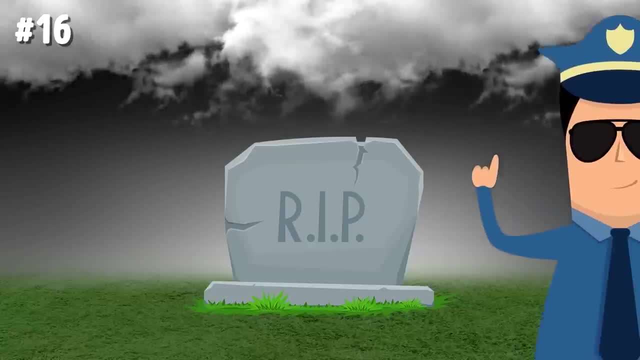 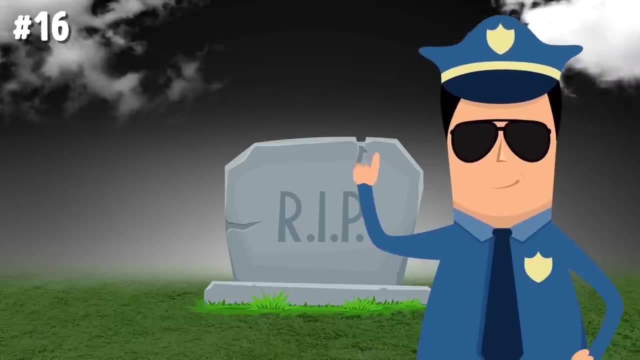 is against the law, right? Well, that's why a living person can't be buried in South Dakota, North Dakota, or anywhere for that matter. Nowhere in the sentence did I say the person had passed away. Therefore, they're still alive and well.